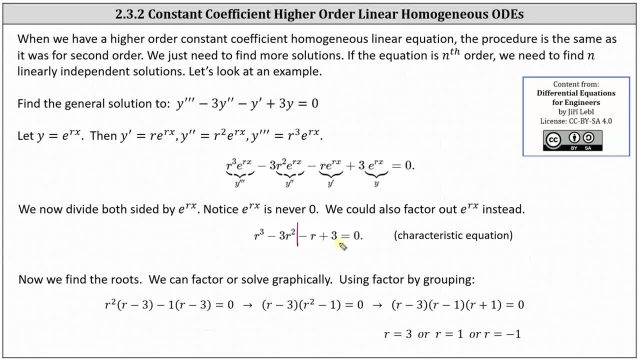 and then we factor out the greatest common factor from the left and right and we should have a common binomial factor, Factoring r squared from r cubed minus three. r squared, we have r squared times the quantity r minus three. Now we have a common binomial factor. 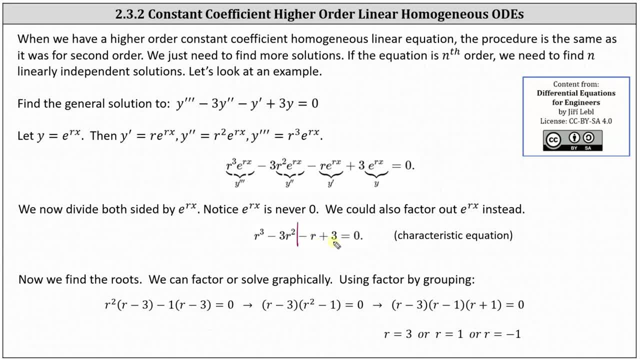 Next we factor out negative one from negative r plus three, which gives us negative one or minus one times the quantity. r minus three equals zero. Notice we do have a common binomial factor of r minus three. We now factor r minus three from the left. 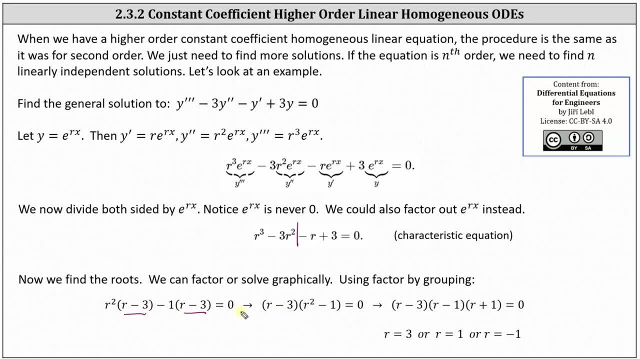 which gives us the quantity r minus three times the quantity r squared minus one equals zero. r squared minus one is a difference of squares, giving us a factor of r minus one and a factor of r plus one. The three roots of solutions are: r equals three. 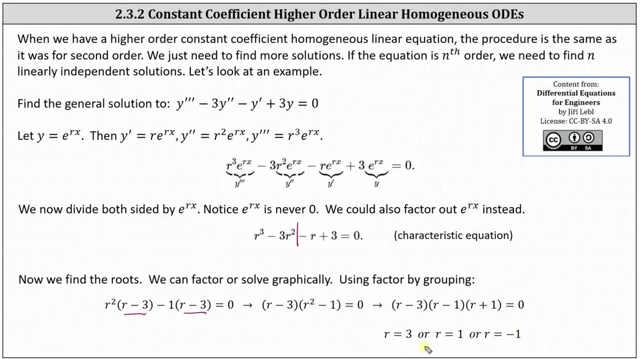 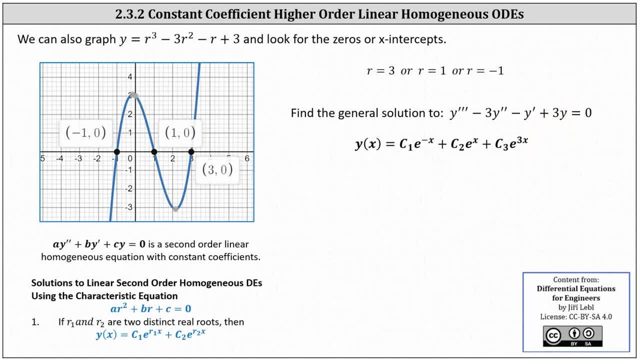 r equals one and r equals negative one. Notice we have three distinct real roots On the left. if we were to graph the characteristic equation, notice how we do have roots of negative one, one and three When we had a second-order linear homogeneous equation. 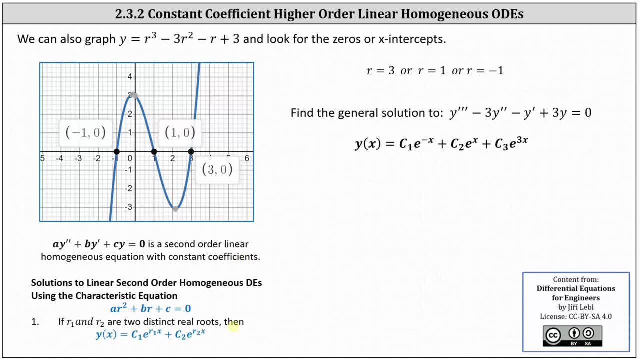 with constant coefficients. recall when we had two distinct real roots. the general solution was: y of x equals c sub one times e to the power of r sub one times x, plus c sub two times e to the power of r sub two times x. 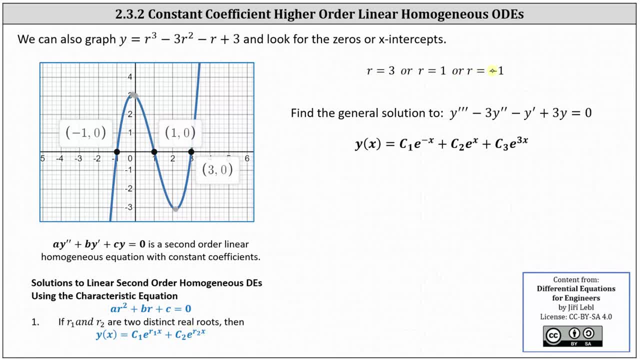 And because we have three distinct real roots, the general solution is: y of x equals c sub one times e to the power of negative x using the root of negative one, plus c sub two times e to the x using the root of positive one. 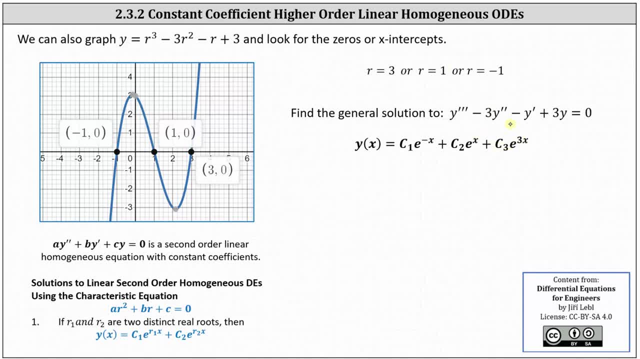 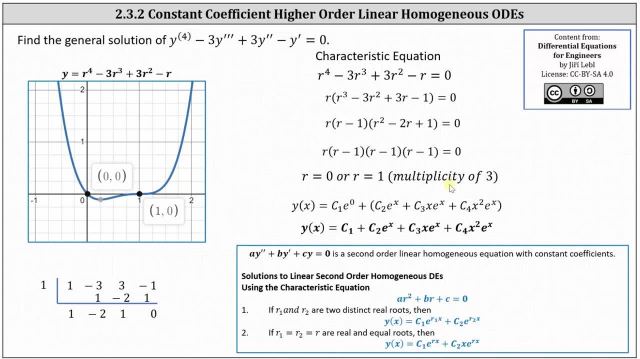 plus c sub three times e to the power of three x, using the root of positive three. Let's look at a second example. Let's find the general solution to the fourth order: constant coefficient, linear, homogeneous differential equation Going straight to the characteristic equation. 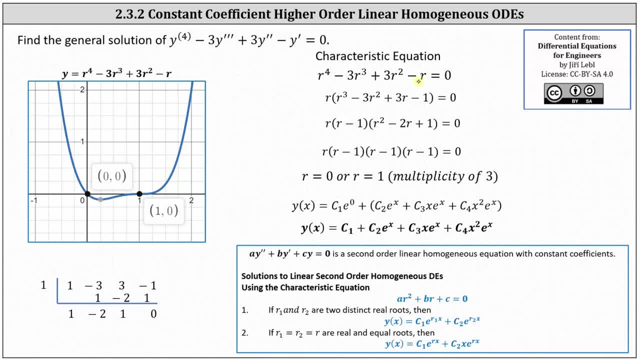 we have r to the fourth minus three. r cubed plus three. r squared minus r equals zero. Notice how we have a common factor of r. Factoring out r gives us this equation, And then from here we need to find one root for r cubed minus three. r squared plus three. r minus one. 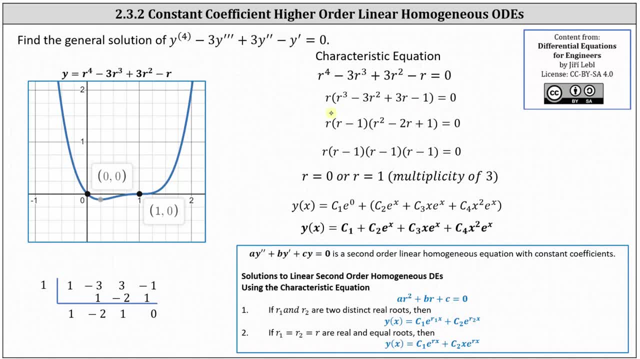 which we can do by analyzing the graph on the left. Notice how the graph on the left does show the root of zero from the factor of r And notice one is also a root which means r minus. one must be a factor of the given degree four polynomial. 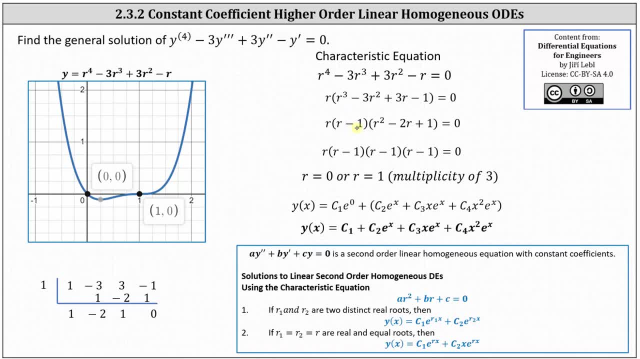 From here we can perform synthetic division, which I've shown here below, where, for r cubed minus three, r squared plus three, r minus one, we have one negative three, three negative one Because one is a root. we have a one here on the left. 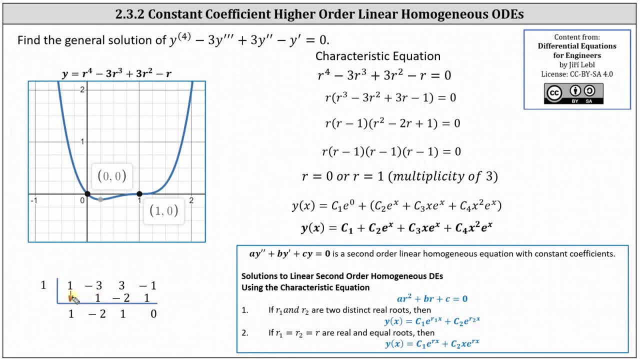 And then we perform synthetic division which for review we bring down the one multiply by the root of one, one times one plus one, and then we add vertically Negative: three plus one is negative two. Multiply by one again, which gives us negative two. 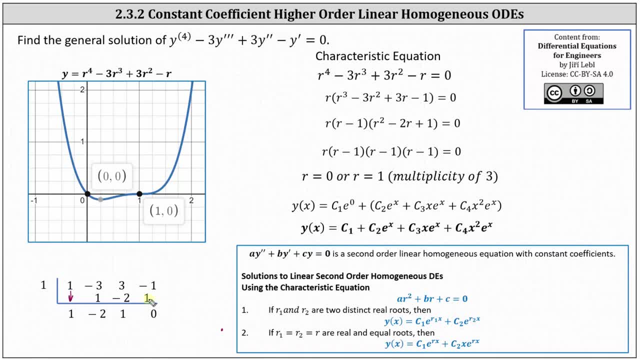 Add, get positive one. Multiply by one. again add, we get zero. The one negative two. one represents the factor of r squared minus two, r plus one, which factors. again, Notice how we have r times three factors of r minus one. 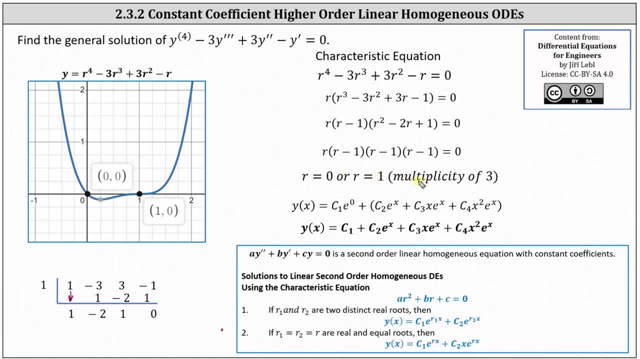 This indicates the roots are zero and one where one has a multiplicity of three. So, again, if we go back two, what we know about second order, constant coefficient, linear, homogeneous differential equations, if we have two real, equal roots, 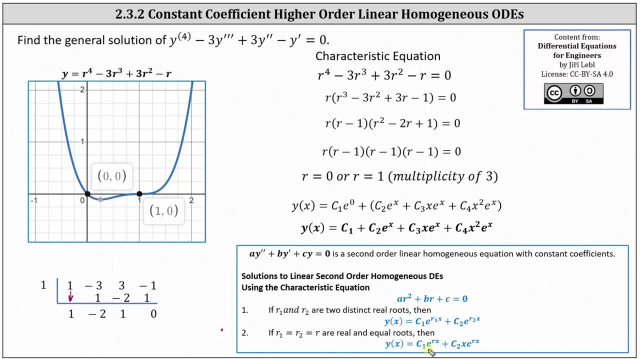 the general solution was: y of x equals c sub one times e to the power of rx, plus c sub two times x times e to the power of rx. So for our general solution we have y of x equals, using the root of zero. 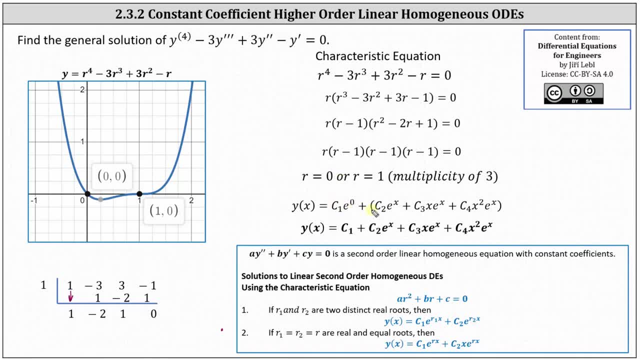 we have c sub one times e to the zero and then plus, because the root of one has multiplicity of three. we have c sub two times e to the x plus c sub three times x, e to the x plus c. sub four times x squared e to the x. 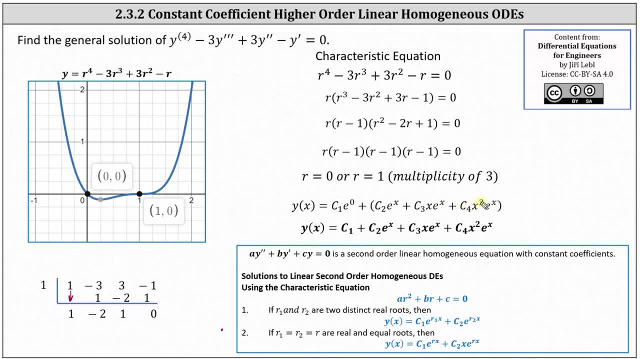 Notice for this third term. here we have two factors of x. Simplifying, we have the general solution of y of x equals c sub one plus c sub two. e to the x plus c sub three. x. e to the x plus c sub four. x squared e to the x. 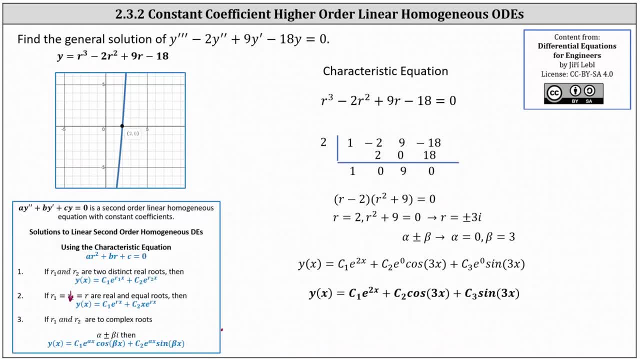 Let's look at one more example where we have complex roots. Let's find the general solution to y triple prime two, y double prime plus nine, y prime minus 18, y equals zero. The characteristic equation is: r cubed minus two r squared. 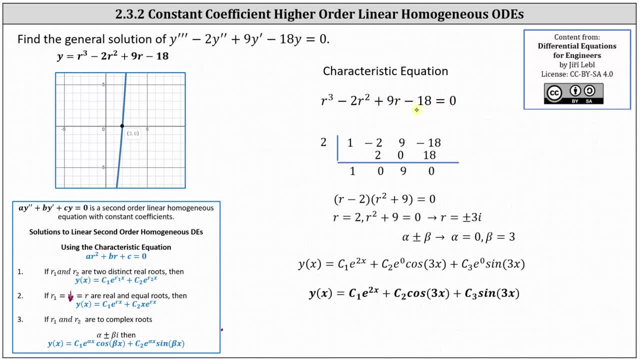 plus nine, r minus 18 equals zero. Analyzing the graph on the left, we can see: one root is r equals two, which gives us a factor of r minus two, And then to determine the remaining factor, we perform synthetic division using two. 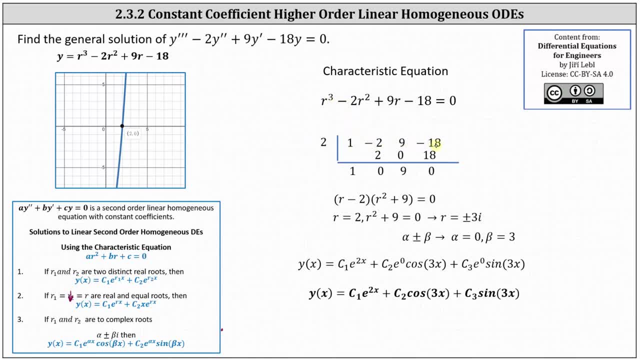 So notice how, again, the coefficients are one negative two nine and negative 18. And the root of two is outside. We bring down the one: multiply by two. add. multiply by two: add. multiply by two: add. 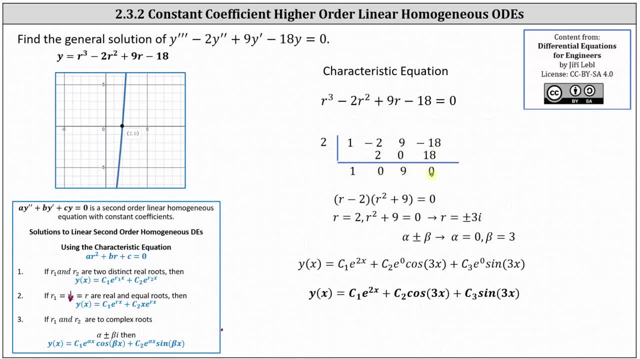 The result is one zero, nine. zero, which indicates the remaining factor is r squared plus nine. So now in factored form we have the quantity r minus two times the quantity r squared plus nine equals zero. This indicates r equals two. 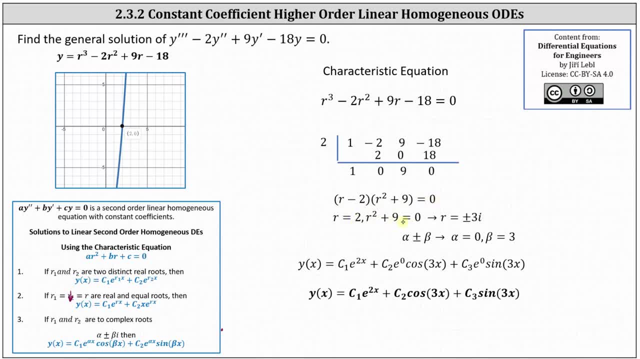 which we already knew from the graph. And then r squared plus nine must equal zero. subtracting nine and square rooting both sides, we get r equals plus or minus three. i Recall when the equation was second order and we had complex roots or complex solutions. 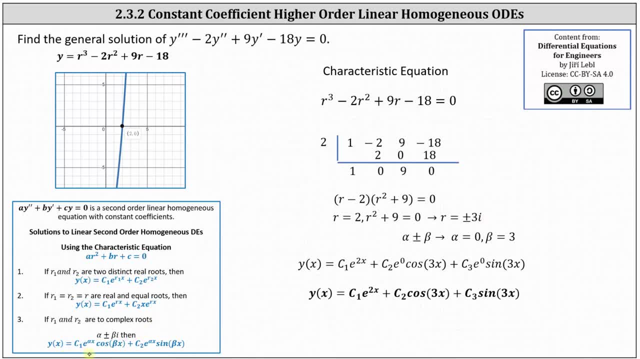 the general solution was in the form of y of x equals c sub one e to the power of alpha x cosine beta x, plus c sub two times e to the power of alpha x times sine beta x, which means our general solution, first using the root of two. 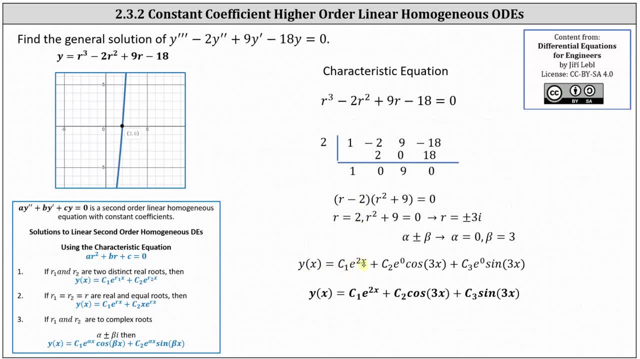 we have y of x equals c sub one times e to the power of two x, and then, using the two complex solutions or imaginary solutions where alpha is zero and beta is three, we have c sub two e to the zero times cosine three x, plus c sub three e to the zero sine three x. 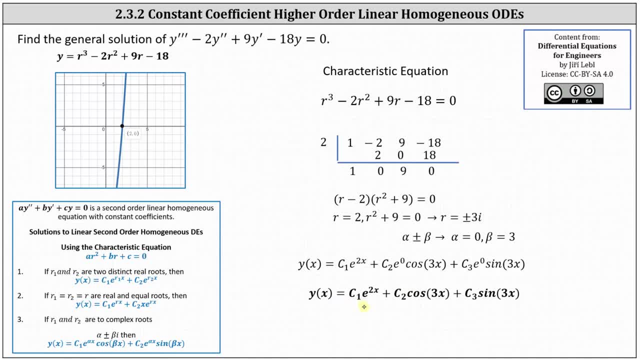 Simplifying, we have the general solution of y of x equals c sub one e to the two x plus c sub two cosine three x plus c sub three sine three x. We'll look at some more examples in the next several videos. I hope you found this helpful. Thank you.